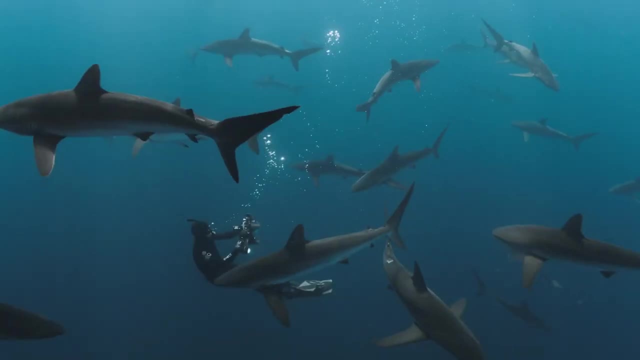 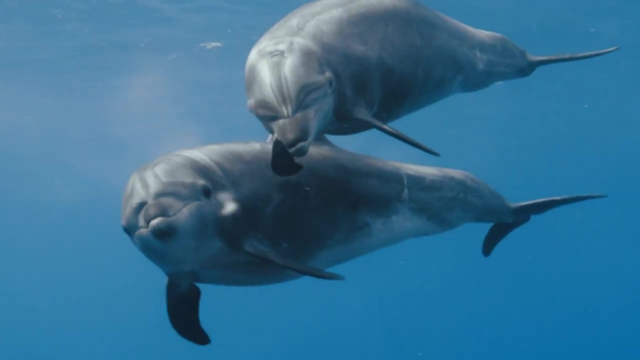 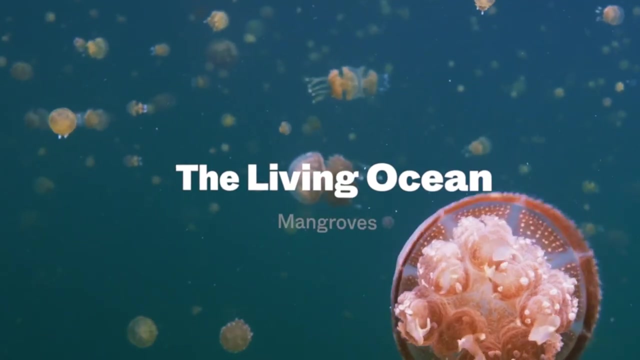 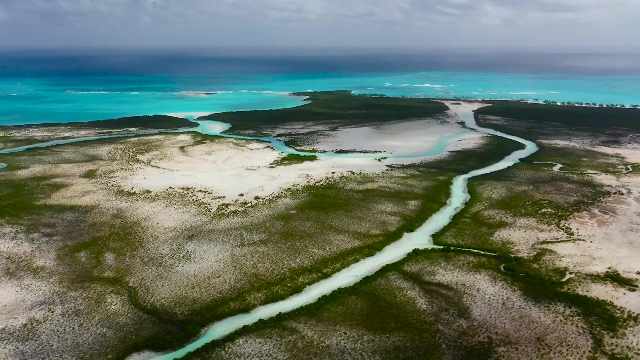 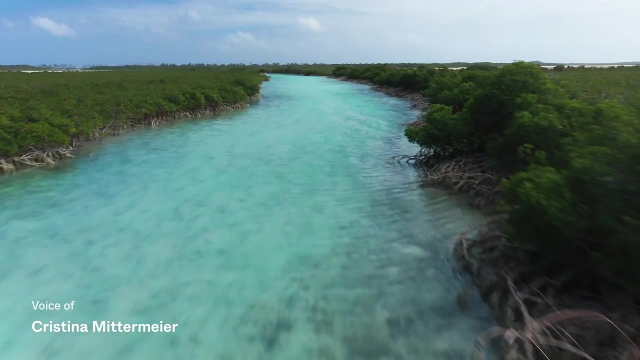 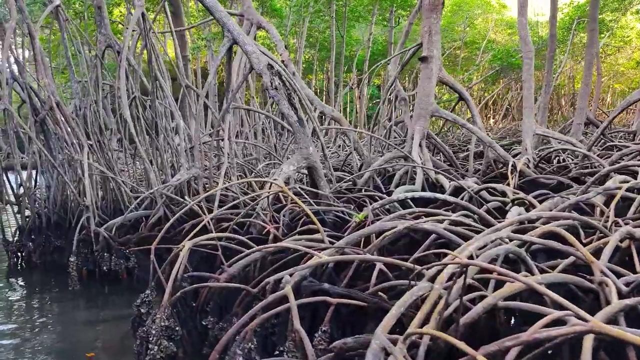 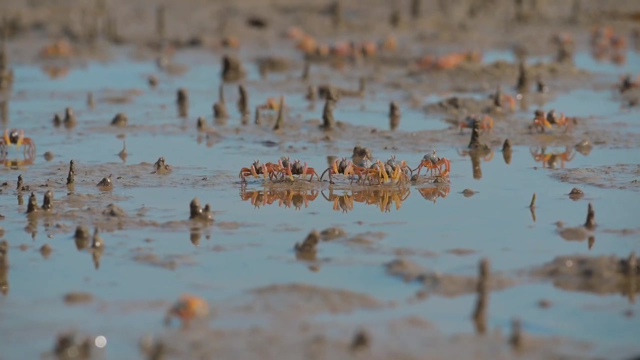 The funny thing is. the funny thing about looking at a mangrove forest is that at first glance it doesn't look like much. It's just a bunch of trees growing in the water. Mangroves are the only trees on this planet that can grow in salt water. 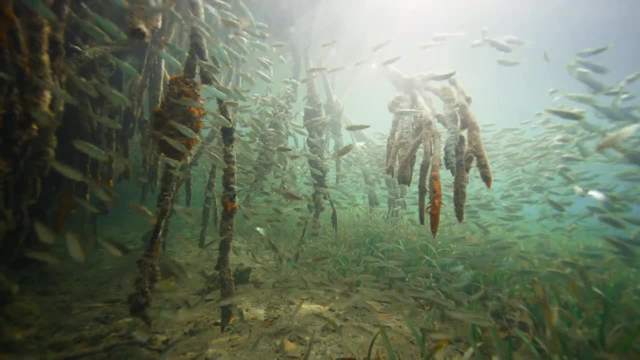 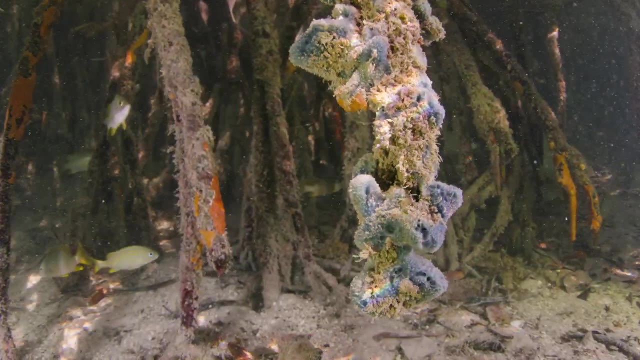 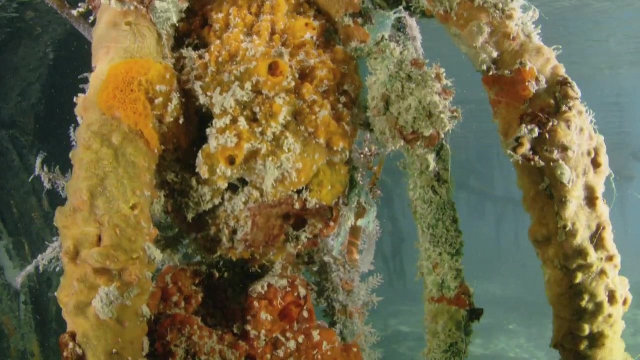 They build a system of elevated roots that are propelling the trees up into the air, but are also reaching deep into the sediment. You'll find corals growing on the roots themselves, And among the maze of roots is the home of so many species. 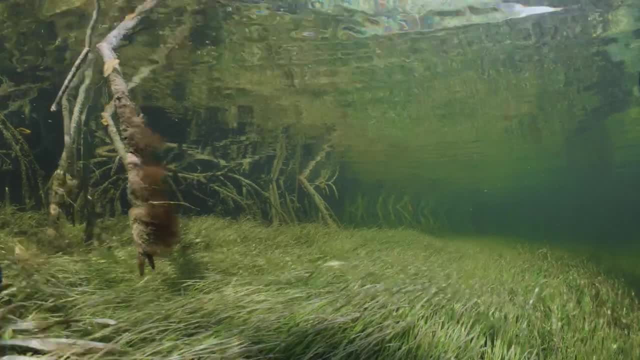 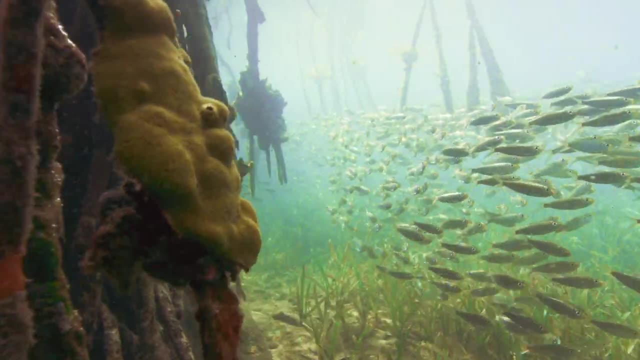 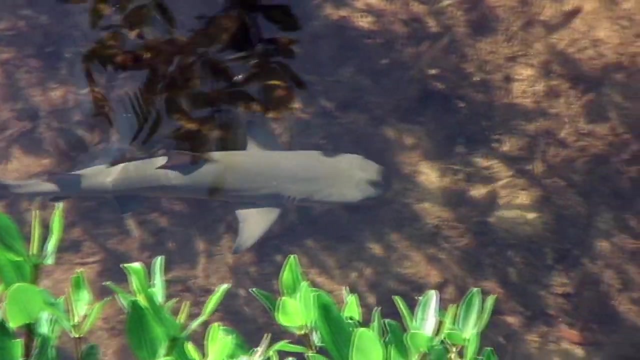 I always love getting in the water and just floating down the mangrove riding the current. It's like a roller coaster. You just never know what you're going to find. Lemon sharks in Bimini start their lives in the mangrove. 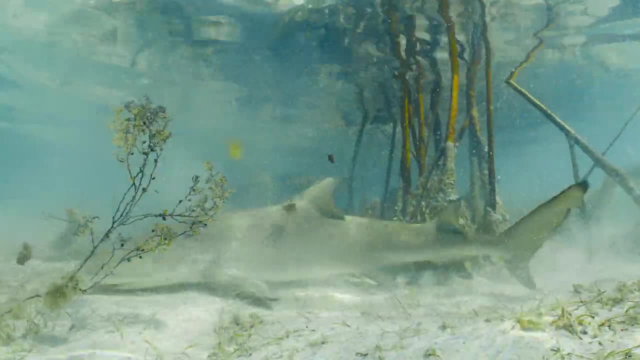 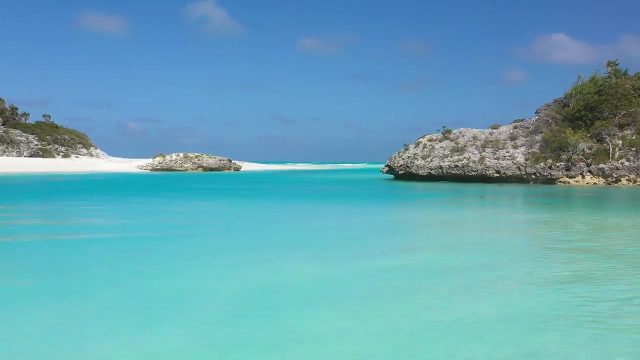 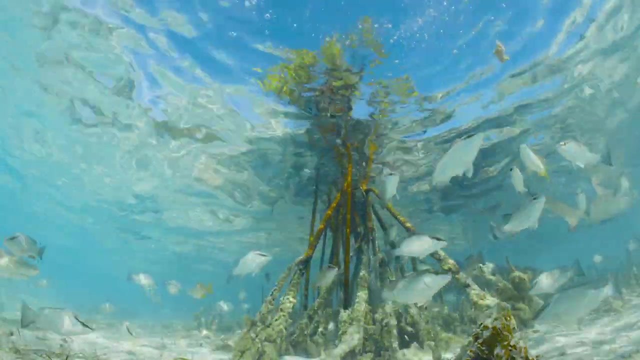 and they spend six years in the mangrove system, hiding from the larger predators, learning how to be sharks and then eventually getting big enough and courageous enough to leave the shelter of the mangrove to go out in the open ocean. Eventually they will return to the same mangrove. 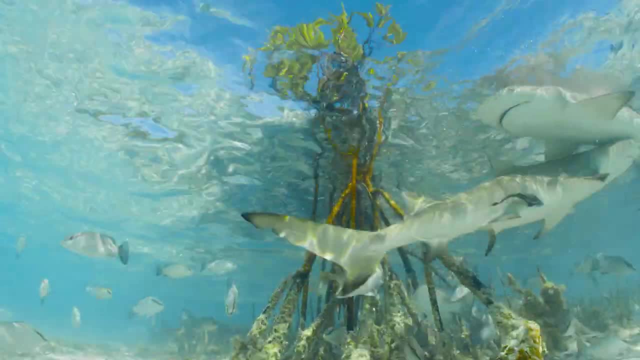 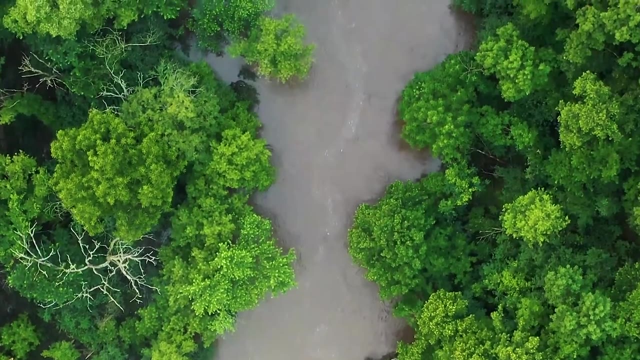 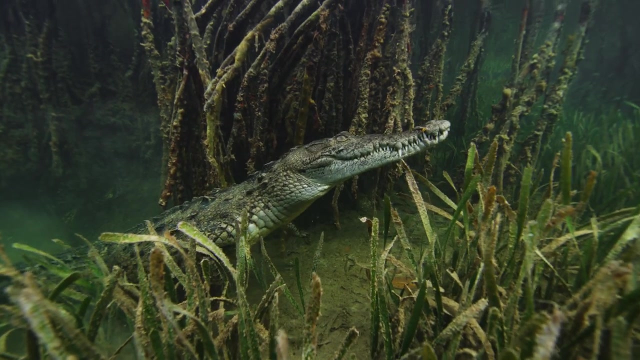 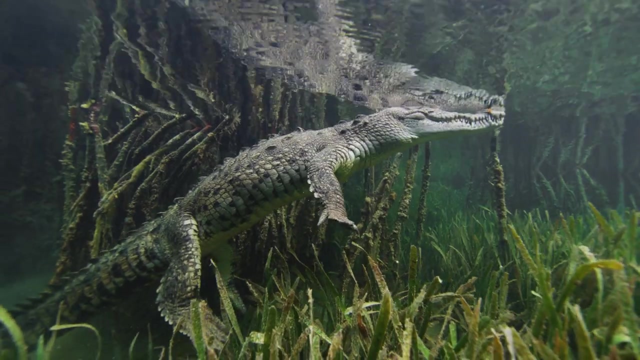 where they were born, to mate and to start the reproduction cycle again. One of my favorite characters to encounter in the mangrove is the crocodile. There's something really primal about coming face-to-face with a crocodile in a mangrove forest- Such a mysterious animal. 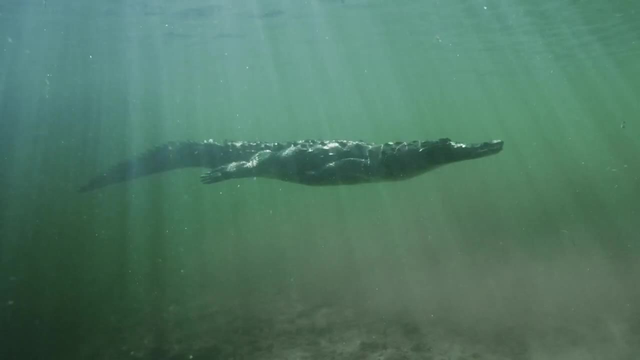 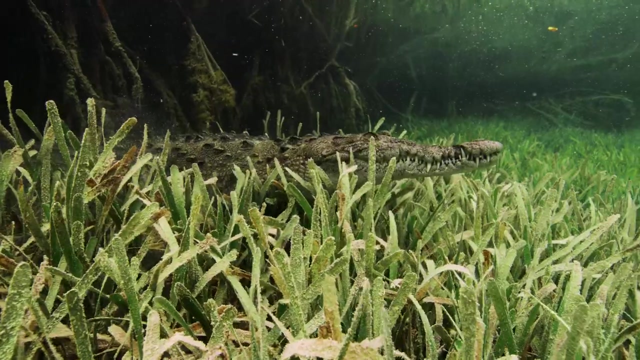 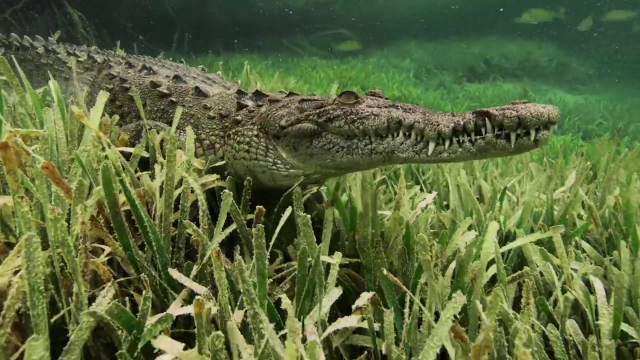 an animal that has survived for millions of years unchanged. It's perfectly adapted to live in a mangrove ecosystem. It can hide, it can hunt. There's just a lot of poetry to these animals. I was so excited to see the crocodile.